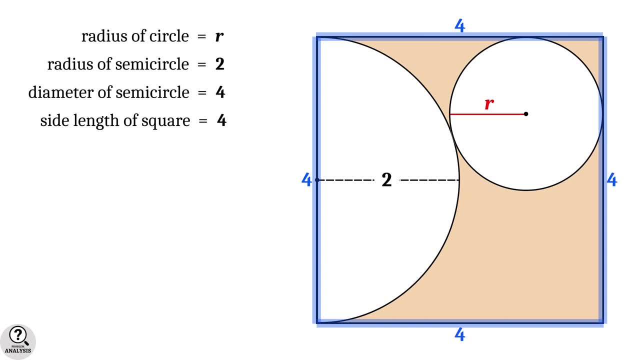 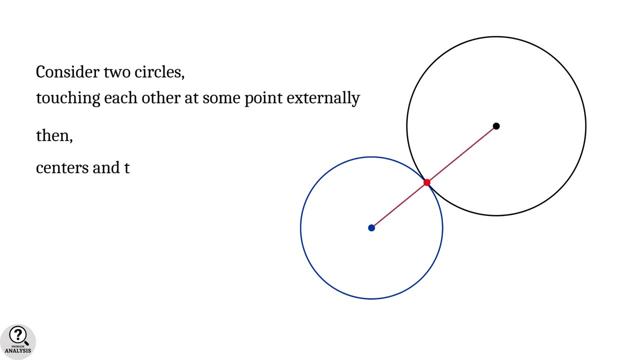 of the square will be 4 units. Now, before going to the further explanation, we need to note an important property of tangent circles. So consider two tangent circles. they are touching each other at some point externally. Then the centers of the circles and their 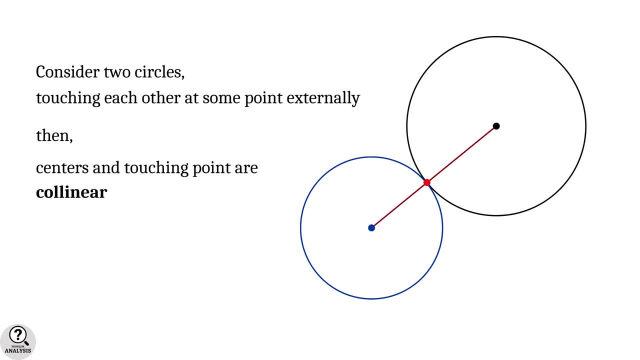 touching point are collinear, That is, lying on the seam line. This is called a diagonal. And if the center of the circles is Movie, then the center of the circles will be up. And if the center of the circles is Linear, this is another tangent circle. If the center 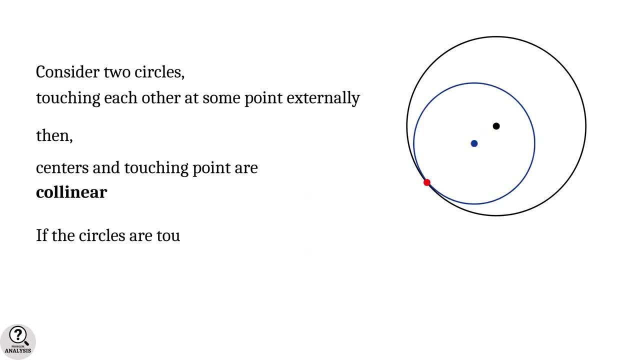 circle is vertical, then the center of the circles will be up. If the center of the circles is Now, if the circles are touching internally, ie one inside the other, still the result is true, That is, centers and the touching point are collinear. 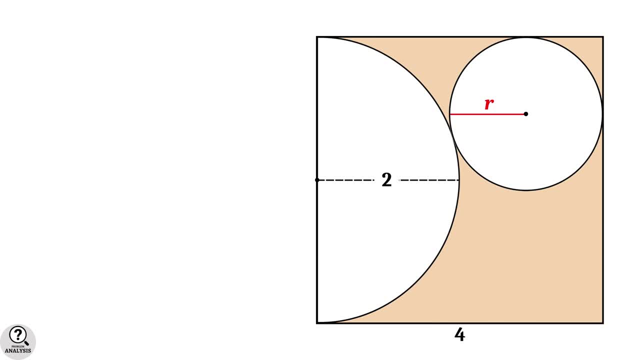 Now come back to the figure. We know that the circle and the semicircle in our diagram are touching each other. Therefore, by the property of tangent circles we mentioned, their centers and the touching point are collinear And in this line, this part is a radius of the circle and so equal to r. 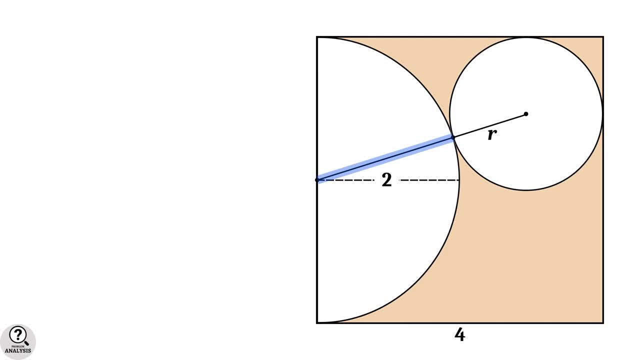 And the remaining part is a radius of the semicircle, which is equal to 2 units. Now draw this perpendicular line to form a right triangle here. Clearly, its hypotenuse is equal to 2 plus r. Now its height is equal to radius of the semicircle, that is, 2, minus this side, which is again. 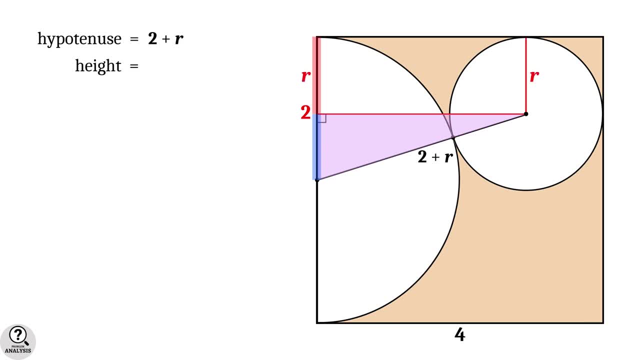 equal to the radius of the semicircle, Then height is equal to 2 minus r. And now the top edge of the triangle is equal to side length of the square, that is, 4, minus this length, which is equal to the radius of the circle, that is r. 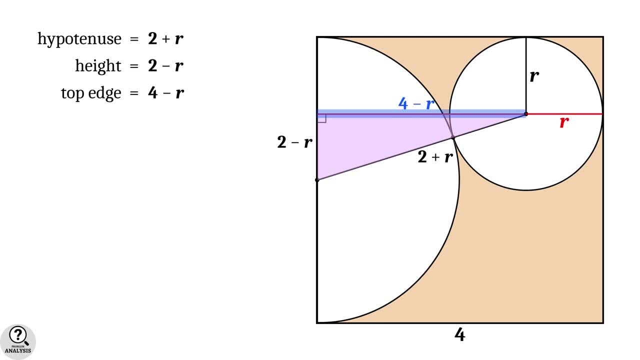 Then the top edge is equal to 4 minus r. Now we can apply the Pythagoras theorem to get r plus 2 whole square is equal to 4 minus r whole square plus 2 minus r whole square. The left hand side expands to r square plus 4r plus 4.. 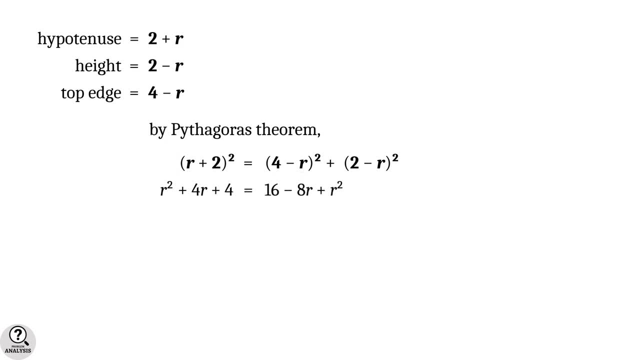 And the right hand side expands to 16 minus 8r plus r square plus 4 minus 4r plus r square. That is equal to 20 minus 12r plus 2r square. And finally it simplifies to r square minus 16r plus 16r. 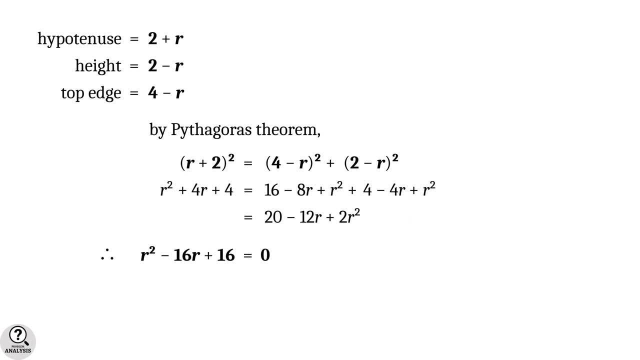 I gently do this. Now, let me simply take this and say that r square is a parallel republic, which implies r square minus 18r is equal to 16r plus 16r 16 is equal to 0, a quadratic equation in R. By solving this equation, we will get the 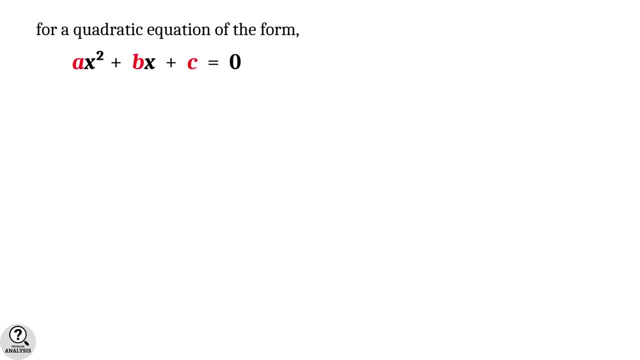 value of R. For a general quadratic equation of the form ax square plus bx plus c equal to 0,. the general solution is given by the quadratic formula, which is: x is equal to minus b plus or minus square root of b square minus 4ac whole divided. 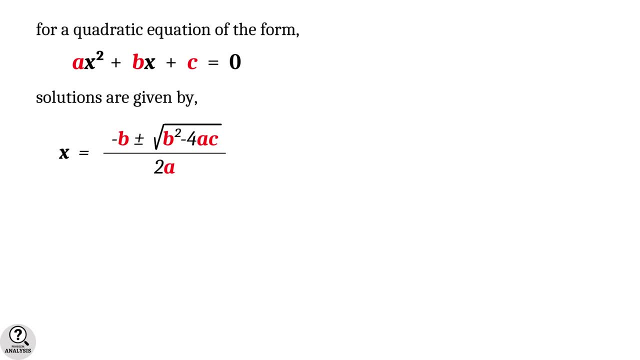 by 2a, And here our equation is: R square minus 16R plus 16 equal to 0.. So, comparing with the general form, we will get a equal to 1,, b equal to minus 16, and c equal to. 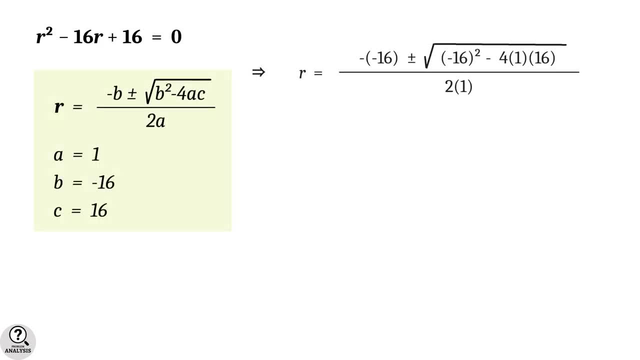 16.. Now substitute these values in the quadratic formula and simplify To get: R is equal to 16 plus or minus square root of 192 whole divided by 2.. That gives R is equal to 8 plus or minus 4 root 3, the two possible values for R. But. 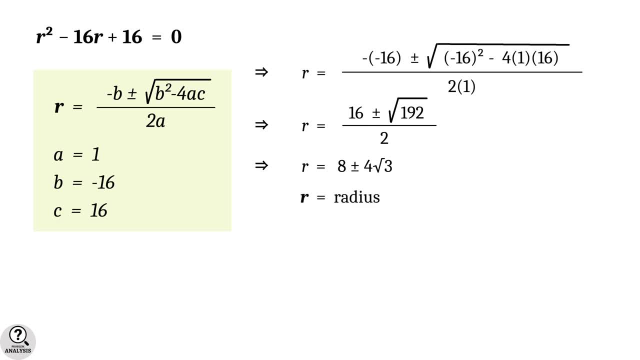 we know that R is the radius of the circle, and so it should be positive. Out of the two values, the value 8 plus 4, root 3, is anyway positive. Now note that 4 into root 3 is approximately equal to 6.928, which is clearly less than. 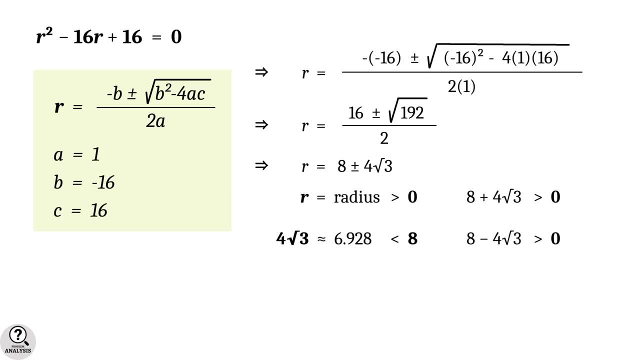 8. And so 8 minus 4 root 3 is also positive. So we need to find which one of these is the suitable value of R. But how to find that? To understand that, come back to the diagram And suppose 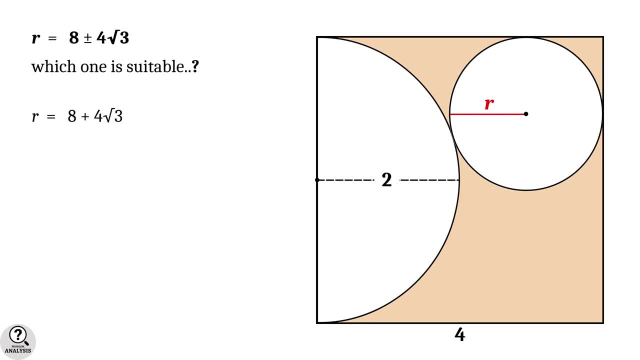 R is equal to 8 plus 4 root 3.. Now remember that R is the radius of the circle, And the circle is lying completely inside the boundary of the square. Therefore, radius of the circle should be less than the side length of the square. 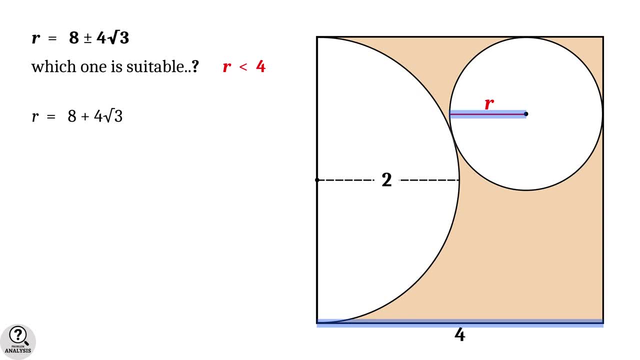 So we can write this as the radius of the circle, And the radius of the circle should be more than 3 paths In fryplane. there, 8 plus 4 root 3 should be the bisschen to the left of R, That is.